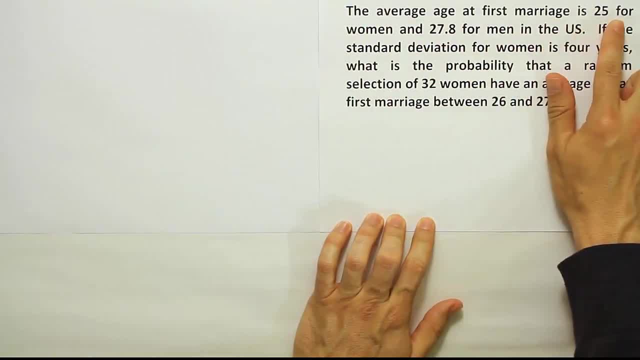 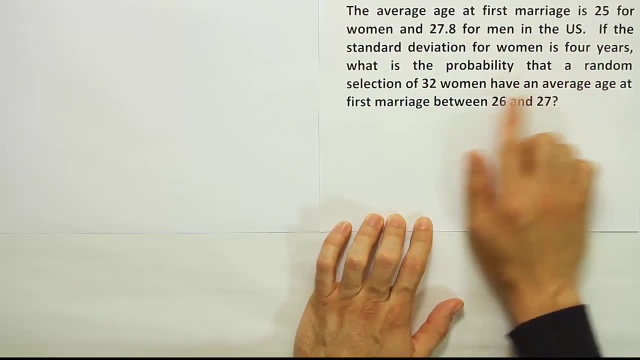 The average age at first marriage is 25 for women and 27.8 for men in the US. If the standard deviation for women is 4 years, what is the probability that a random selection of 32 women have an average age at first marriage between 26 and 27?? 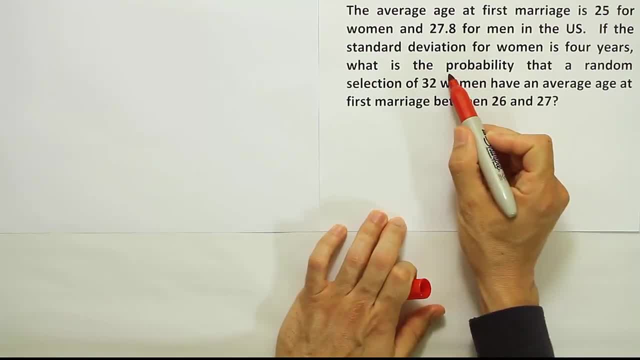 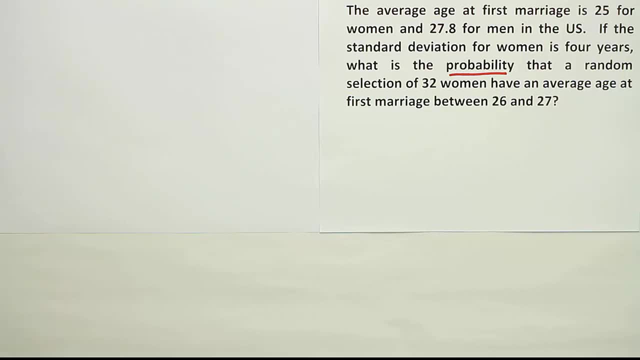 Okay. so the first key phrase I see here is: what is the probability? So I know I'm working on a probability problem. If it's a probability problem, the next question I want to ask is: what's the distribution? Is it bell shaped in distribution? And when I read through this: 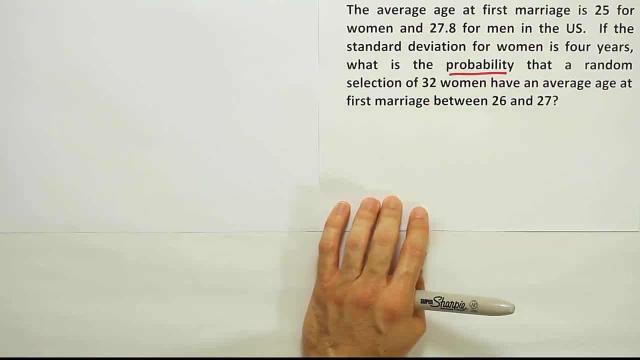 I don't see anything about that. I don't see anything about normally distributed. So I want to look to see if there's another way around that issue, Because it would be nice if it was normally distributed. Then we could do our bell curve and use the bell curve to find the solution. But I do see this: that it's the probability that a random selection of 32 women. 32 women have an average age at first marriage between 26 and 27.. So they're looking for the average to be between 26 and 27.. 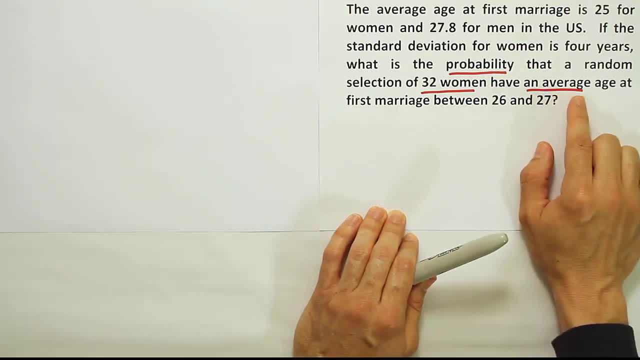 Okay, Okay. This problem is a probability problem about an average, An average that's derived from 32 women. Well, an average for 32 women is X bar, right, That's? in this case, they're talking about X bar. for a group of 32 women, It's X bar. if it's an average, that's from. 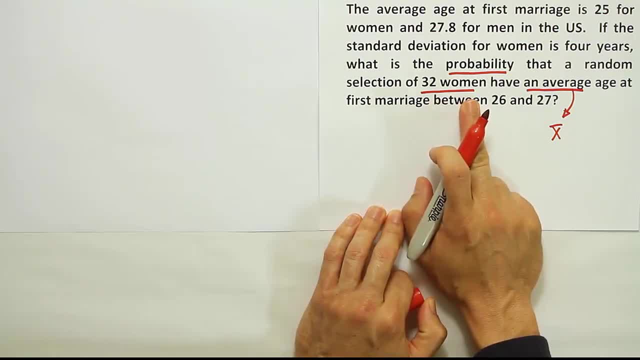 a sample right And 32 women clearly is not the population of women, So I know that it's not mu right. This average is not mu, It's, it's the X bar right For the 32 women And 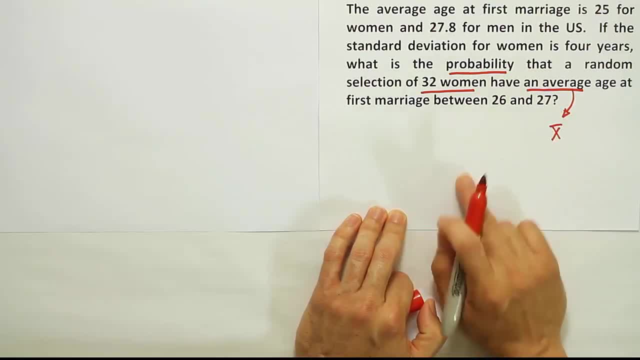 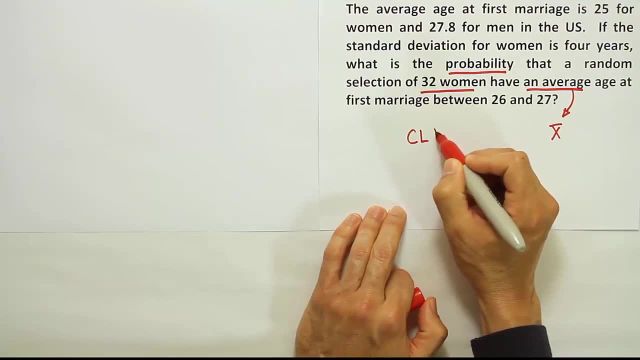 they're asking: what's the probability that that average would be between 32 and 27,, given the other information in the problem? Well, if we're dealing with X bar, we have something called the central limit theorem And that tells me that, essentially, X bar is normally distributed, or at least approximately. 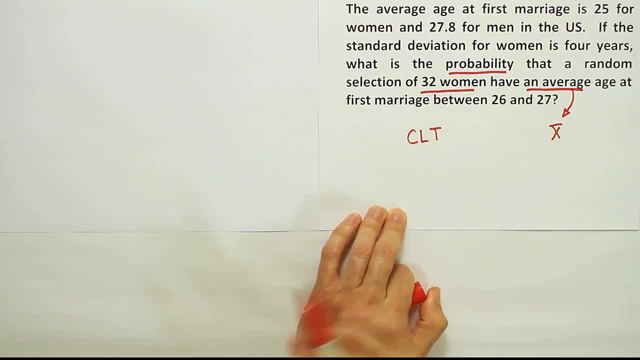 normally distributed when the sample size is greater than 30. So if I see this sample size of 32, it's an indication to me that if the problem is about X bar, I can use the bell curve, And that's really the whole thing here. 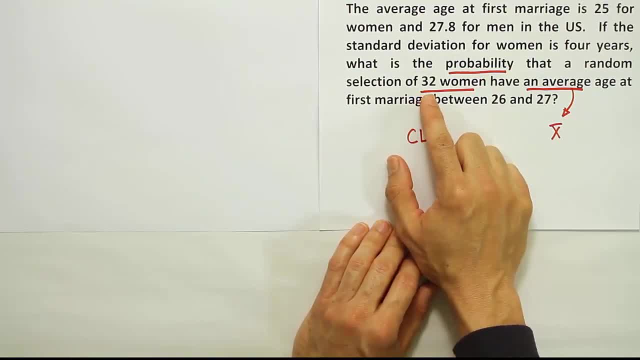 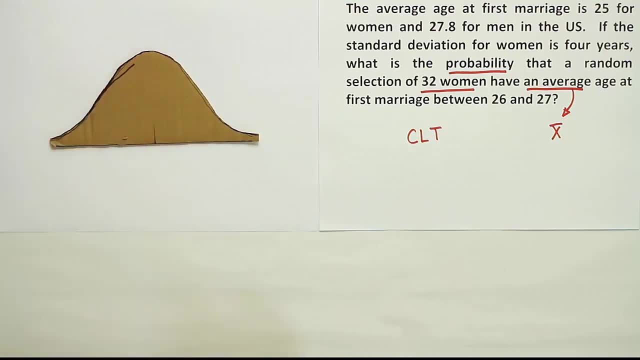 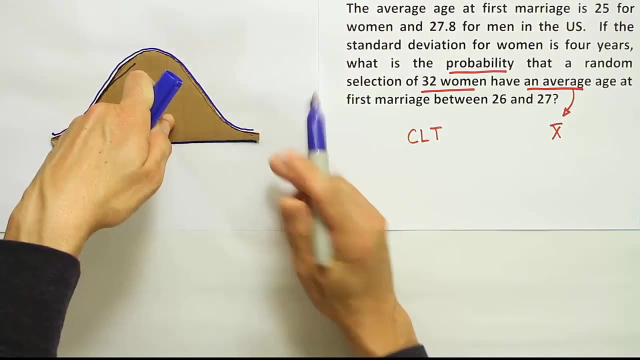 So basically we have a probability problem and we have a sample size greater than 1.. So in this case I can do the bell curve safely. So let's go ahead and do that. I'll put my little bell curve tool up. tool up here, Sorry. Draw the bell curve And now. 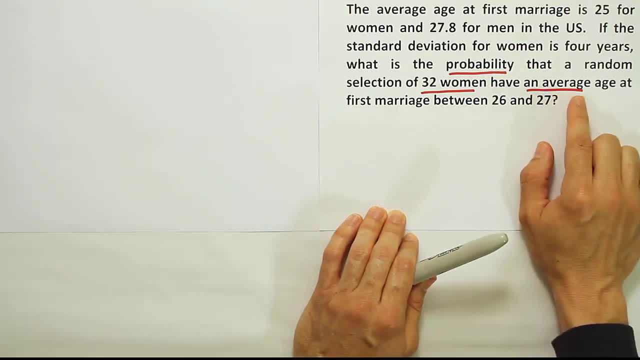 Okay, Okay. This problem is a probability problem, about an average, an average that's derived from 32 women. Well, an average for 32 women is X bar, right, That's? in this case, they're talking about X bar. for a group of 32 women, It's X bar. if it's an average, that's from. 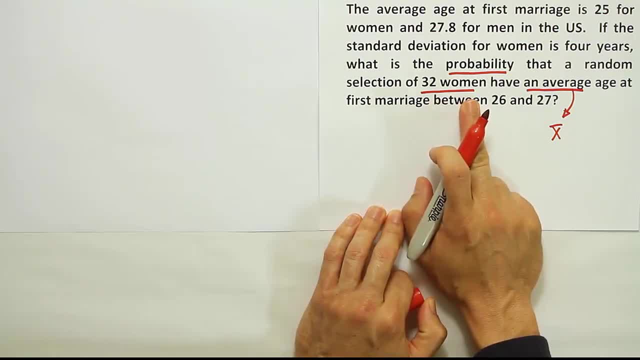 a sample right And 32 women clearly is not the population of women, So I know that it's not mu right. This average is not mu, It's, it's the X bar right For the 32 women And 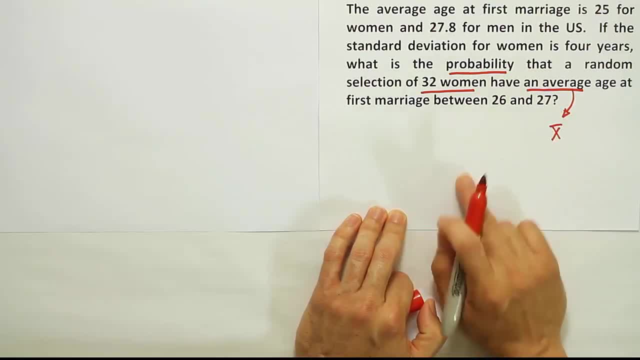 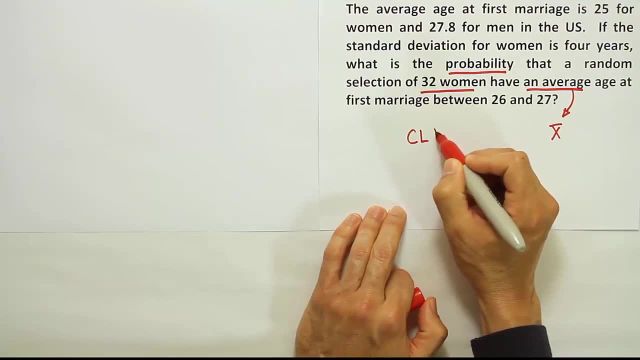 they're asking: what's the probability that that average would be between 32 and 27,, given the other information in the problem? Well, if we're dealing with X bar, we have something called the central limit theorem And that tells me that, essentially, X bar is normally distributed, or at least approximately. 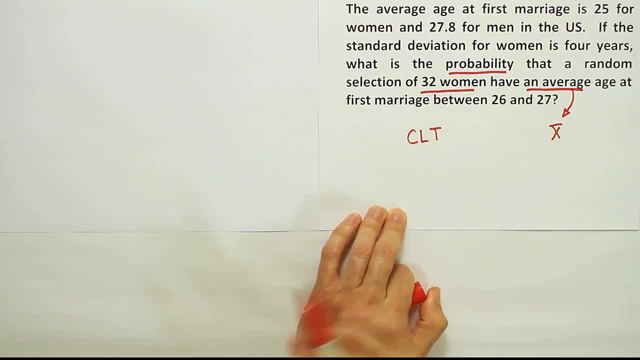 normally distributed when the sample size is greater than 30. So if I see this sample size of 32, it's an indication to me that if the problem is about X bar, I can use the bell curve, And that's really the whole thing here. 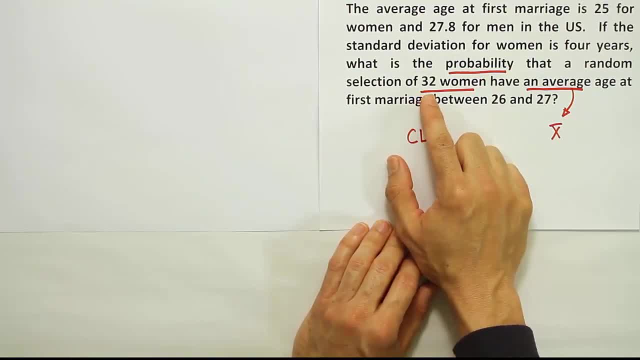 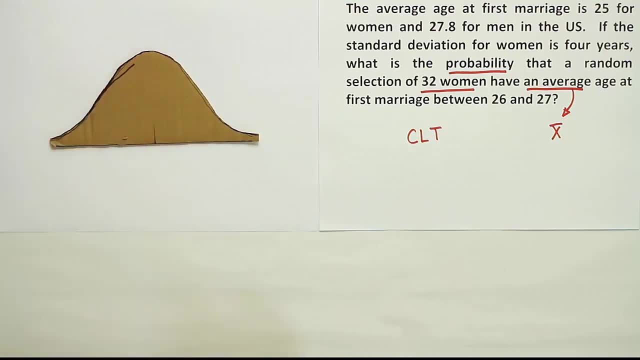 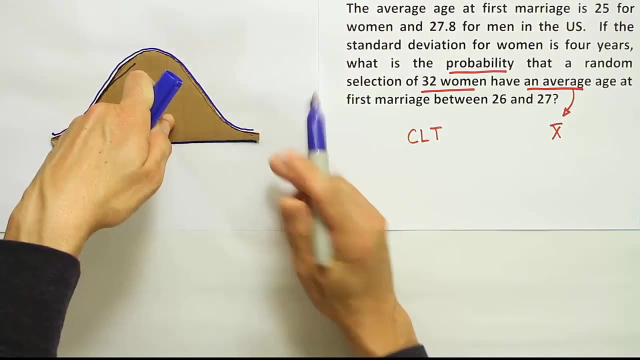 So basically we have a probability problem and we have a sample size greater than 1.. So in this case I can do the bell curve safely. So let's go ahead and do that. I'll put my little bell curve tool up. tool up here, Sorry. Draw the bell curve And now. 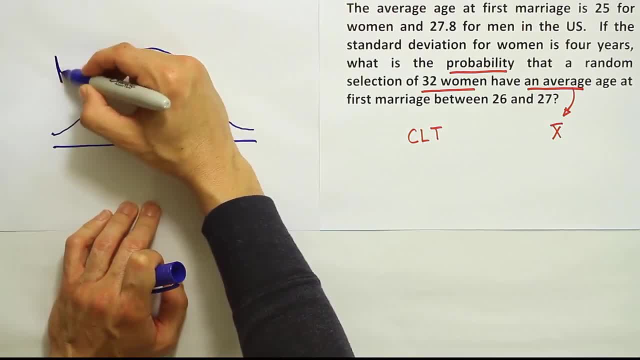 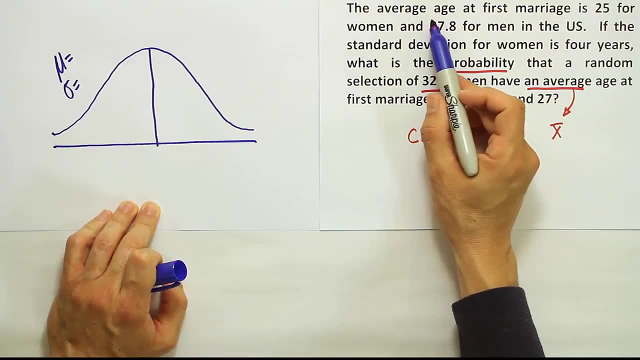 label, its mean standard deviation, et cetera. So when we come to this part of it, you know if I just went through the problem, I'd say: well, they told me that. what the average age at first marriage is: 25 for women, 27.8 for men. So I have two averages here. Which one's? 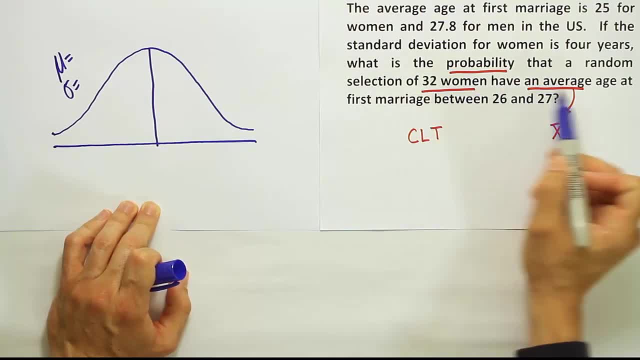 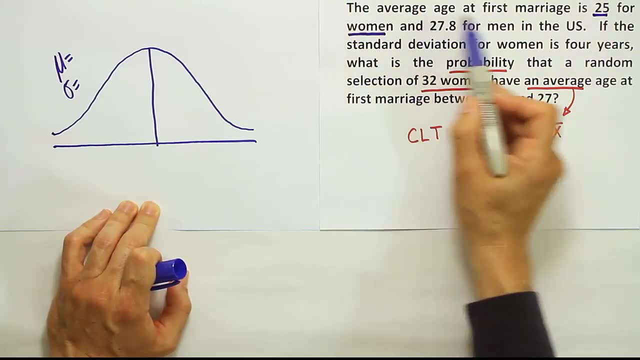 important for us. We're talking about 32 women and dealing with their average, So certainly I'm interested in the women more than the men here. So I'm going to look for the 25, right. The average age at first marriage is 25 for women, So I'm going to put 25 here. 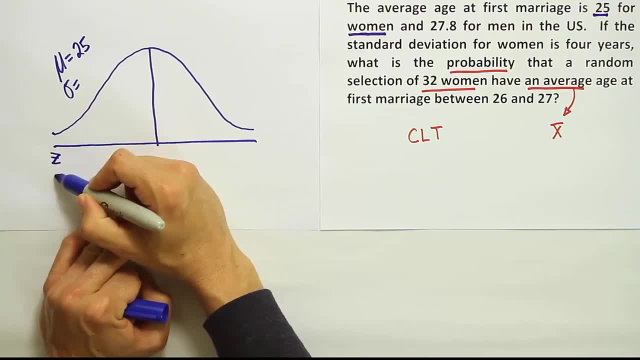 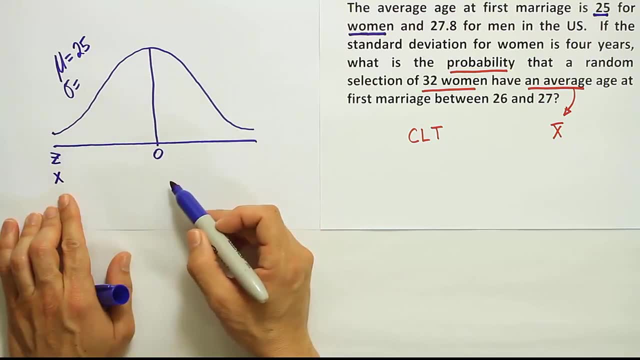 I want to be careful now. This problem is not about X, like we normally have. We normally have a Z axis, zero, and then an X axis where X represents the value for an individual right, So it might be an individual woman's age at marriage right. 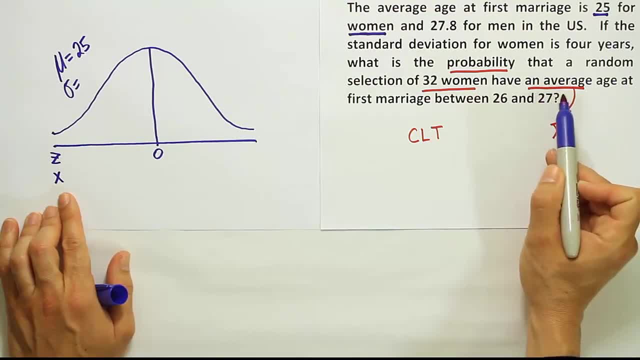 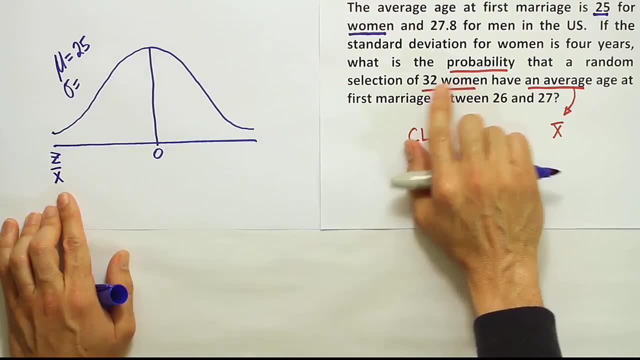 But here we're talking about a sample of 32 women and we're talking about the average being between two numbers. So it's not X that we're dealing with, It's X bar. actually. We see that because it doesn't say the probability that a random selection or a randomly selected 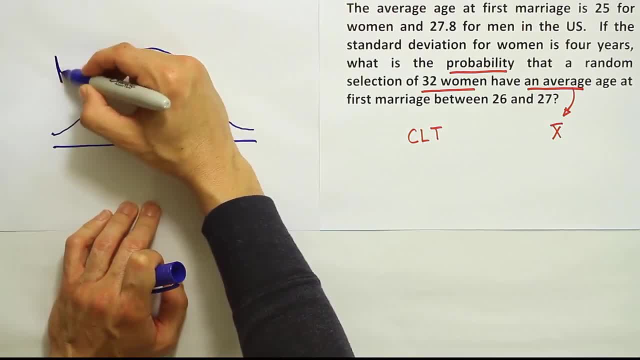 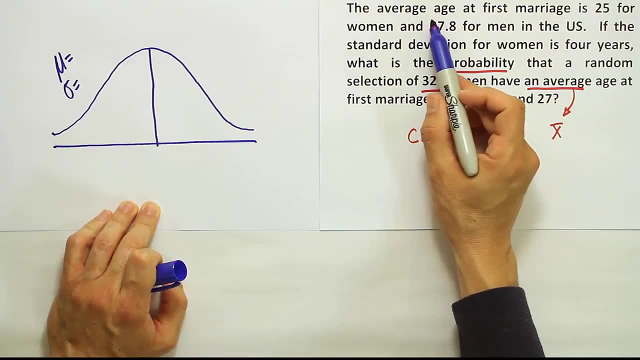 label, its mean standard deviation, et cetera. So when we come to this part of it, you know if I just went through the problem, I'd say: well, they told me that. what the average age at first marriage is: 25 for women, 27.8 for men. So I have two averages here. Which one's? 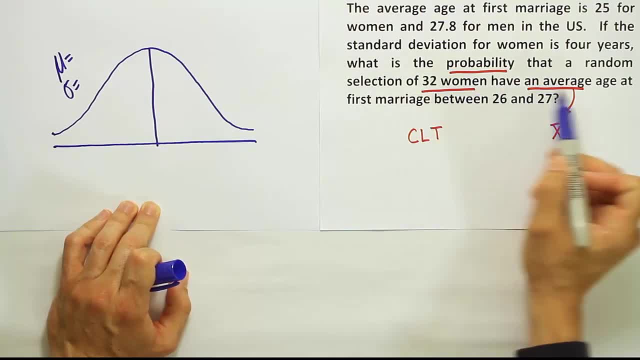 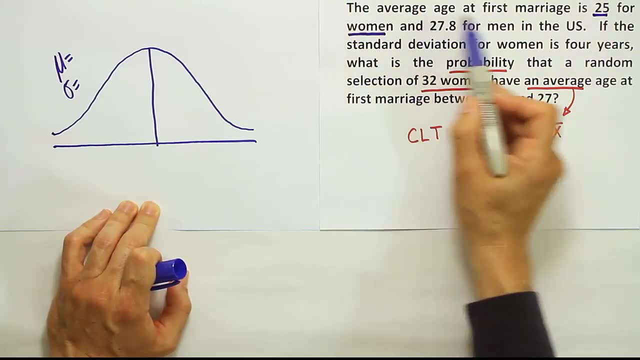 important for us. We're talking about 32 women and dealing with their average, So certainly I'm interested in the women more than the men here. So I'm going to look for the 25, right. The average age at first marriage is 25 for women, So I'm going to put 25 here. 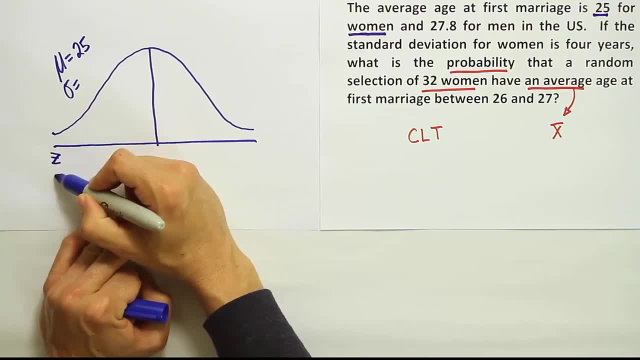 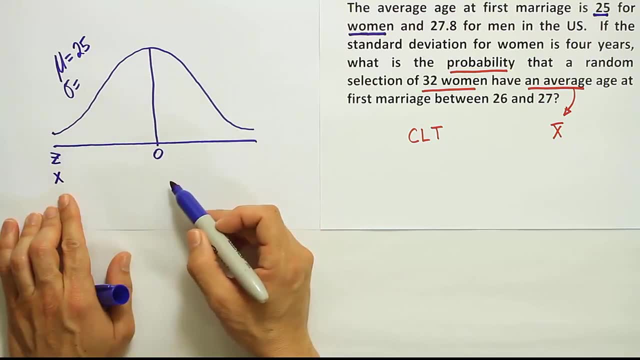 I want to be careful now. This problem is not about X, like we normally have. We normally have a Z axis, zero, and then an X axis where X represents the value for an individual right, So it might be an individual woman's age at marriage right. 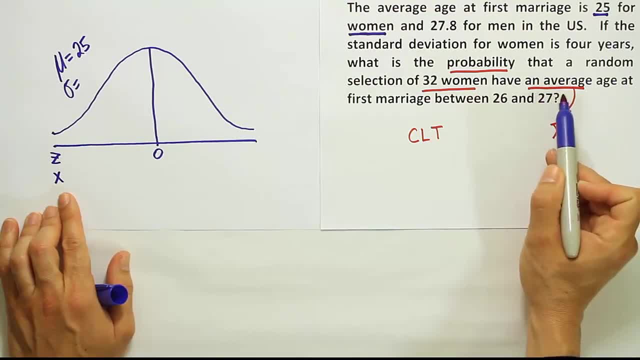 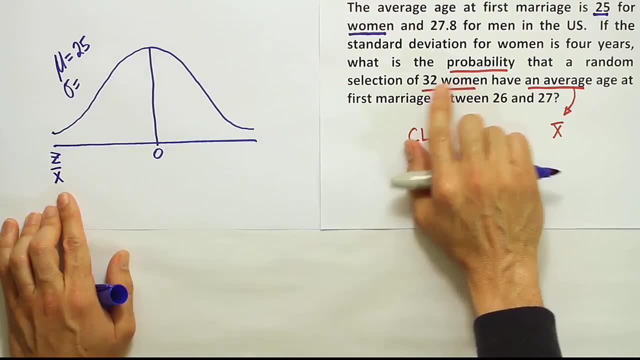 But here we're talking about a sample of 32 women and we're talking about the average being between two numbers. So it's not X that we're dealing with, It's X bar. actually. We see that because it doesn't say the probability that a random selection or a randomly selected 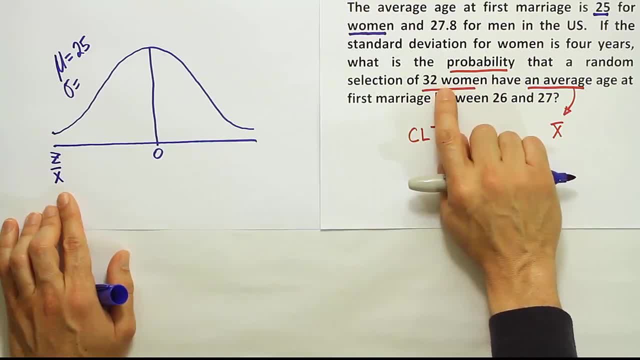 woman. right, It doesn't just say woman, as in one woman, It says 32 women. So that's an important key phrase. You have to pay attention to that. when the problems say what's the probability? in this section, You want to be watching to see if it's the probability that. 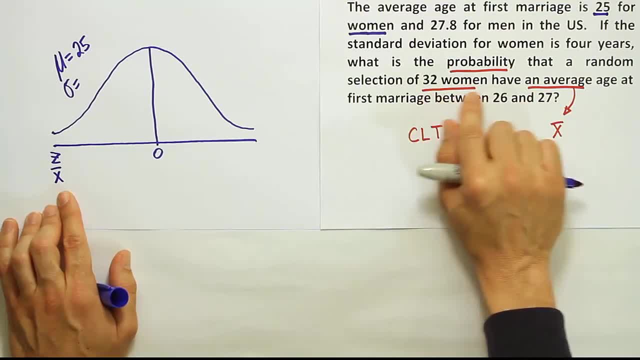 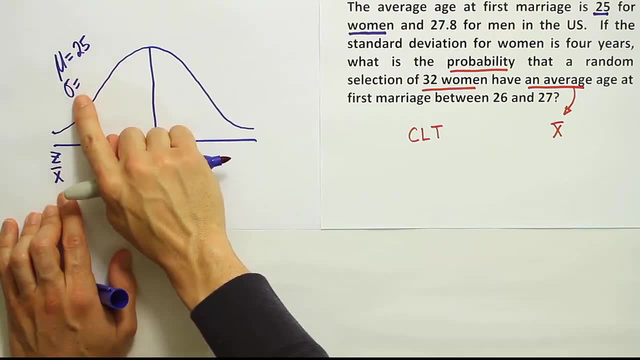 a single woman has an average age between these two numbers, or whether it's more than one woman. If it's more than one woman, you know that this is X bar. That also means that this has to be the mean for X bar And that'll mean that this is the standard deviation for X. 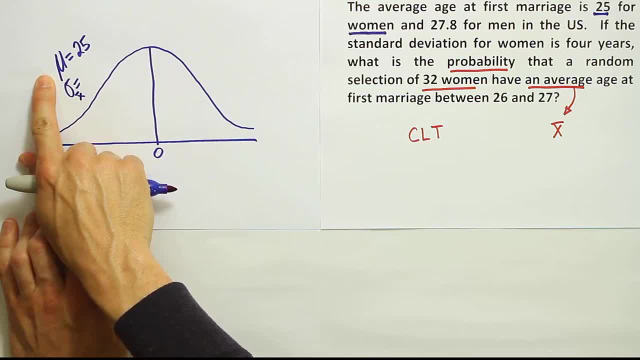 bar. Now, when it comes to the mean, it doesn't matter because the mean doesn't change. The mean for X bar is the same as the mean for the original data set. So it'll be 25 no matter what. But we have to be careful here, and this is the major change in the problem. The 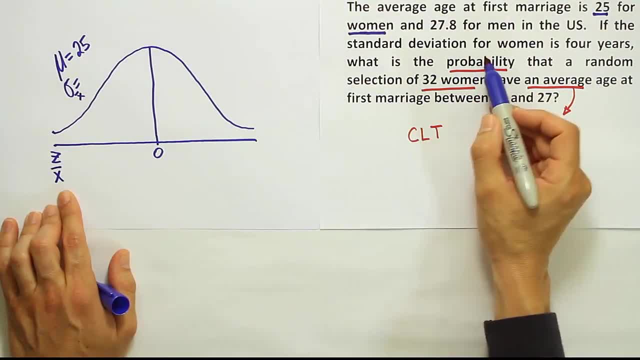 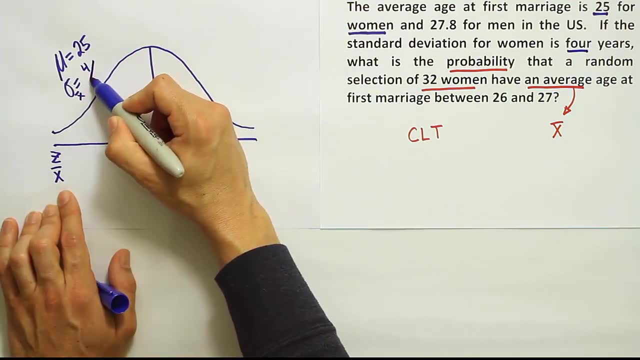 only difference here is that when we go to get the standard deviation, they said: if the standard deviation for women is four years, so we know that it's going to be four. normally it will no longer be four for women, So we're going to have to divide it by the square root of n, So we're adjusting it In. 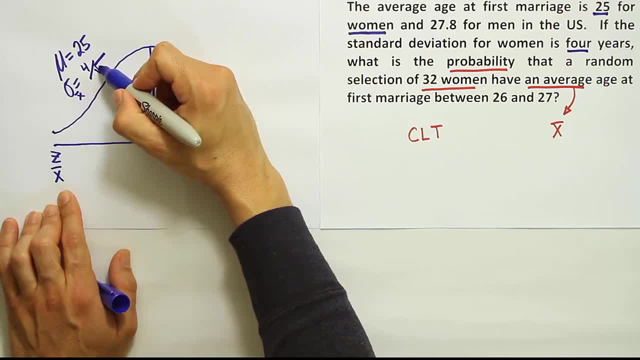 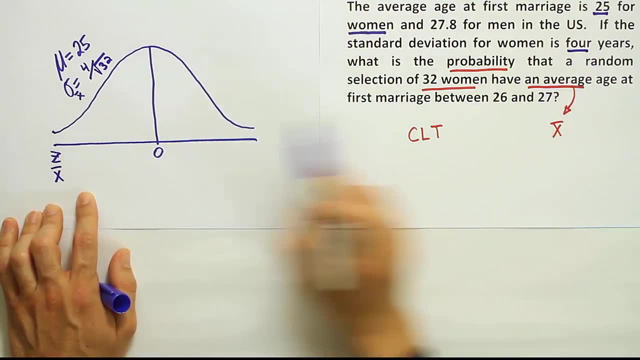 this case the n in this problem is 32.. So we're going to divide by the square root of 32.. So this is the big difference: that when we do the standard deviation we have to take the one they give us, the number they give us, and divide it by the square root of n. 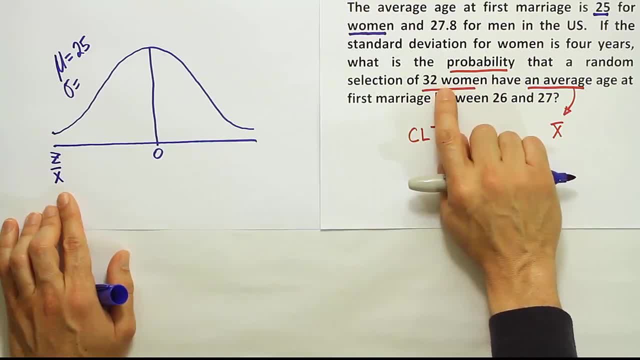 woman. right, It doesn't just say woman, as in one woman, It says 32 women. So that's an important key phrase. You have to pay attention to that. when the problems say what's the probability? in this section, You want to be watching to see if it's the probability that. 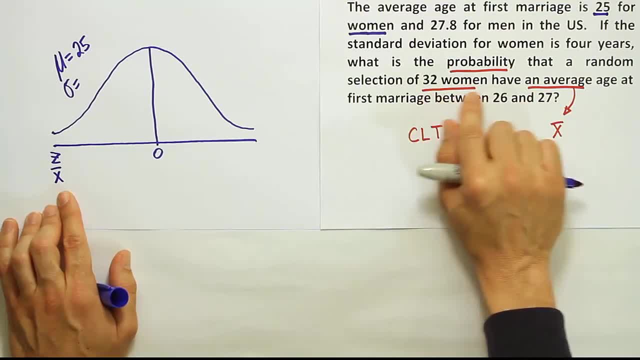 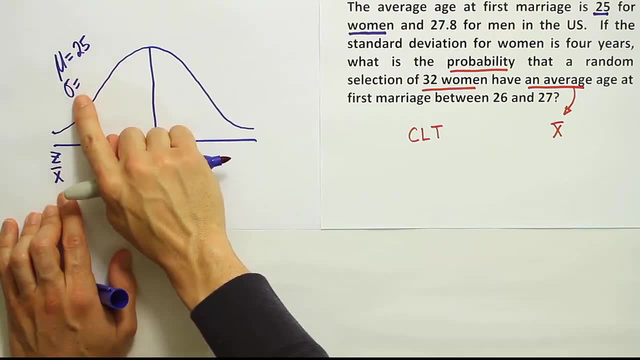 a single woman has an average age between these two numbers, or whether it's more than one woman. If it's more than one woman, you know that this is X bar. That also means that this has to be the mean for X bar And that'll mean that this is the standard deviation for X. 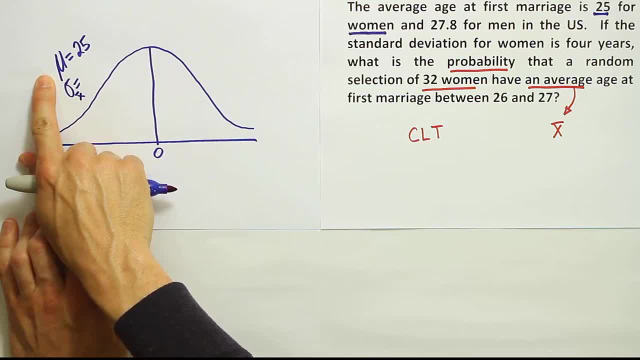 bar. Now, when it comes to the mean, it doesn't matter because the mean doesn't change. The mean for X bar is the same as the mean for the original data set. So it'll be 25 no matter what. But we have to be careful here, and this is the major change in the problem. The 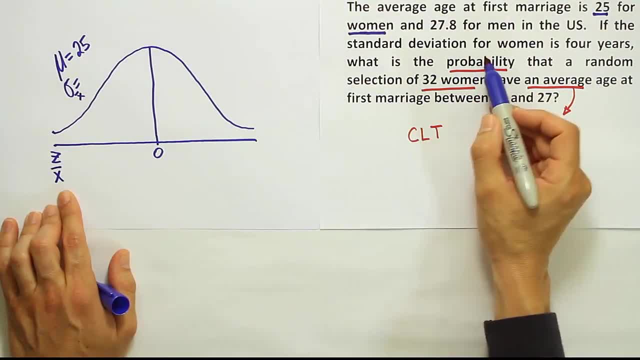 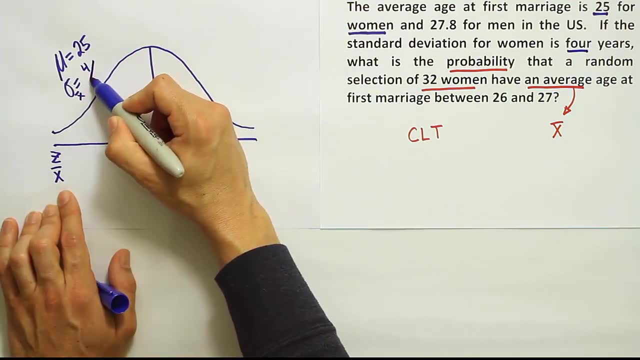 only difference here is that when we go to get the standard deviation, they said: if the standard deviation for women is four years, so we know that it's going to be four. normally it will no longer be four for women, So we're going to have to divide it by the square root of n, So we're adjusting it In. 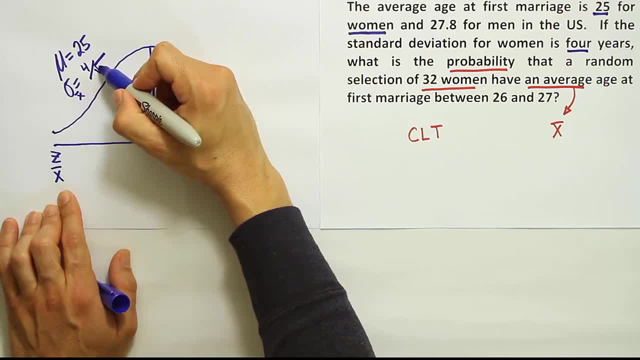 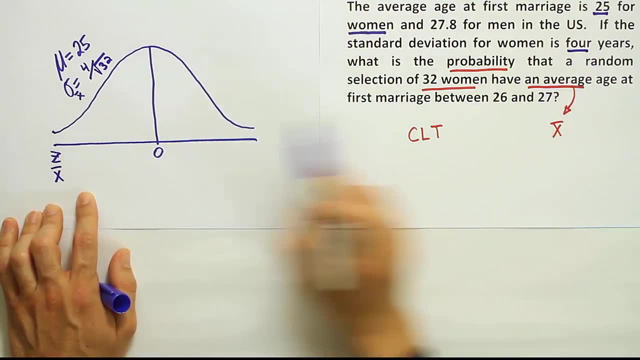 this case the n in this problem is 32.. So we're going to divide by the square root of 32.. So this is the big difference: that when we do the standard deviation we have to take the one they give us, the number they give us, and divide it by the square root of n. 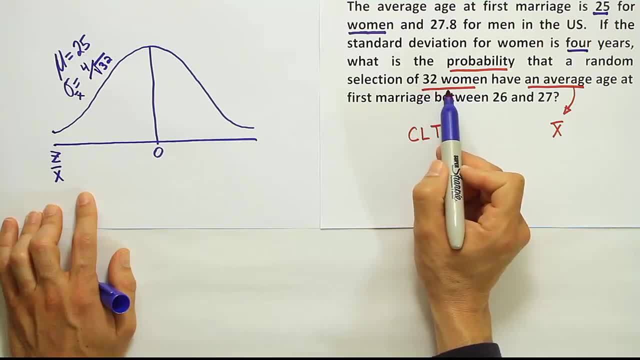 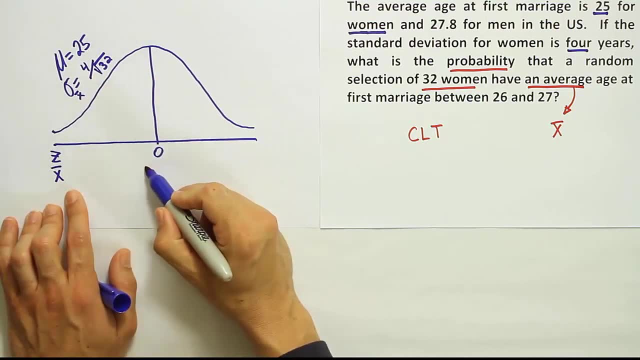 because there is a sample size here. It's not one woman, It's 32 women. So we have to put that into the problem And that's going to change things, of course. All right, So the mean is at 25.. 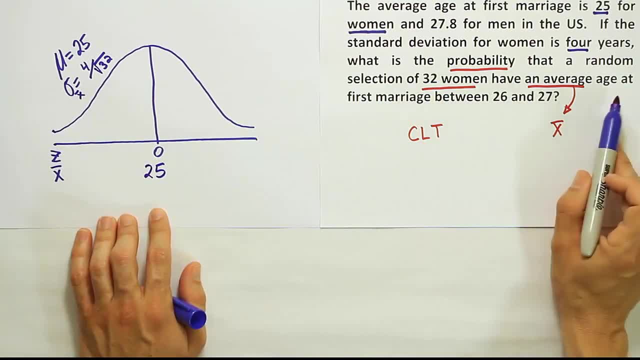 And then we're going to put the two numbers together And then we're going to put the three numbers they asked about. It says the probability that women will have an average age at first marriage between 26 and 27.. So 26 is on the right of 25.. 27 is on the right. 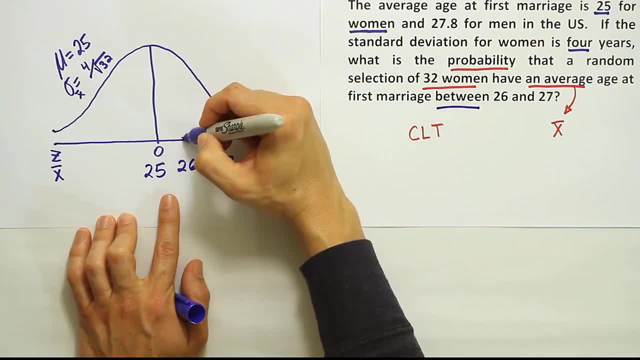 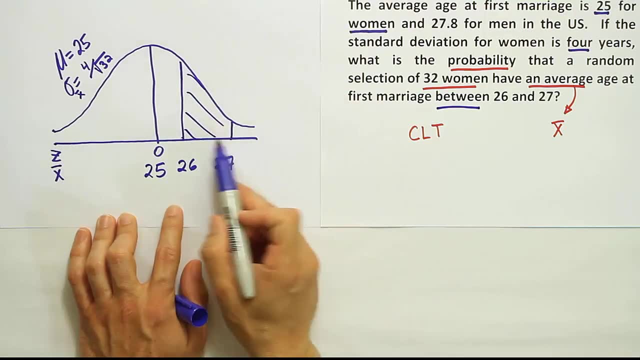 of that And we're talking about between those two numbers. So I'm going to go ahead and draw lines on the curve where those numbers exist and then shade in between to represent the area that I'm looking for. So I'm looking for this area in between. 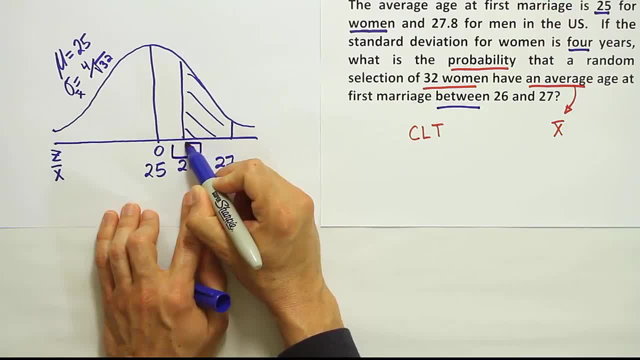 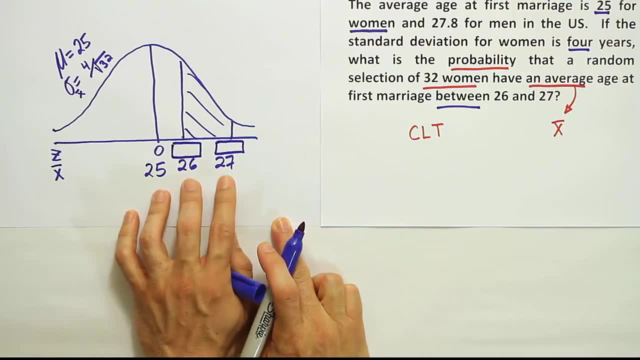 So my goal next is to go to my z table. Remember, once I have my drawing done and it's shaded, I'm supposed to go to my z table, But I can't go there until I have z scores to look up. I can't look up these ages. They're not z scores, So I have to convert them first to 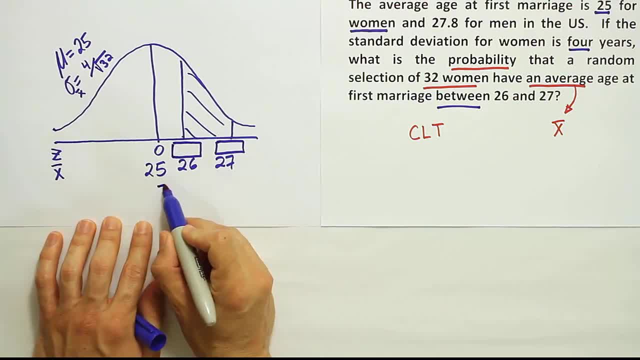 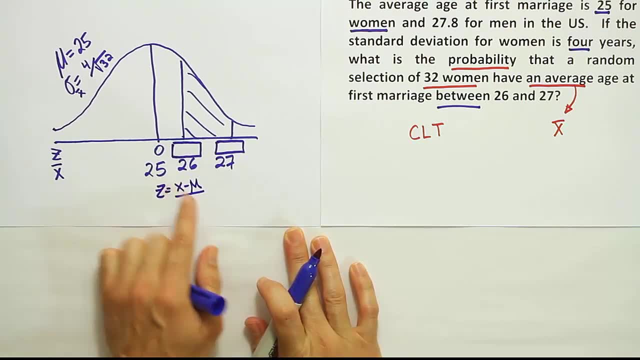 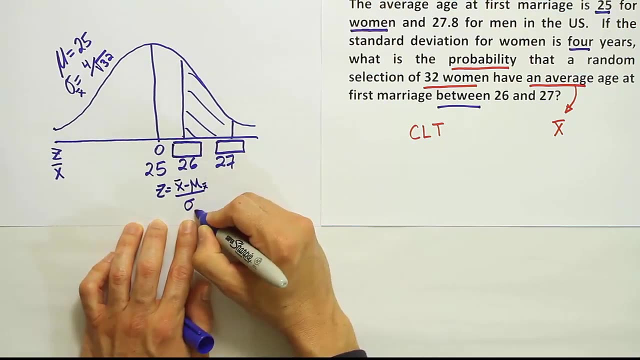 z scores. So let's do that first for the 26.. Remember that z is equal to x minus the mean over sigma, right? Well, here we have x bar minus the mean for x bar, minus sigma of x bar. But that's really just notation, right? I mean, you can plug that stuff in, But essentially 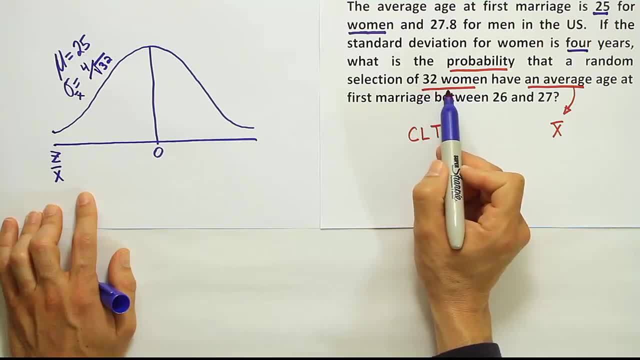 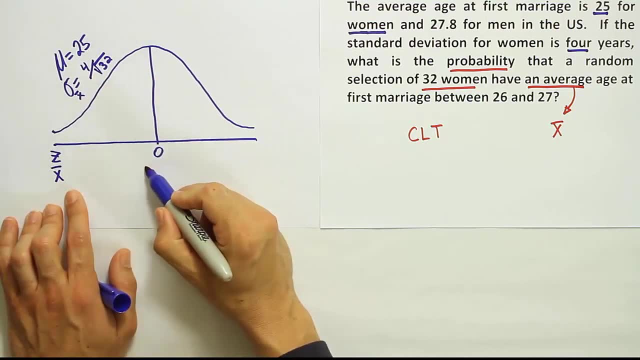 because there is a sample size here. It's not one woman, It's 32 women. So we have to put that into the problem And that's going to change things, of course. All right, So the mean is at 25.. 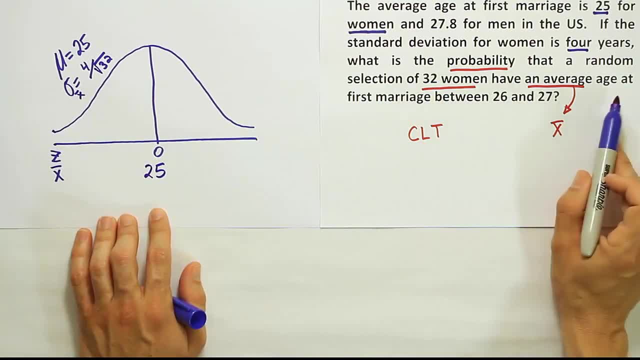 And then we're going to put the two numbers together And then we're going to put the three numbers they asked about. It says the probability that women will have an average age at first marriage between 26 and 27.. So 26 is on the right of 25.. 27 is on the right. 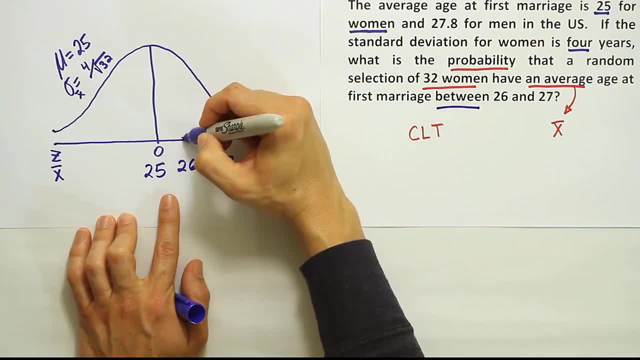 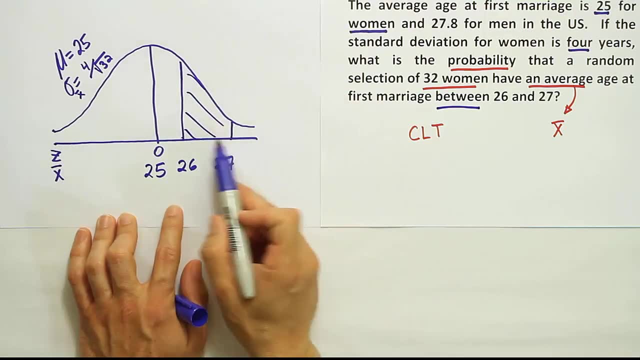 of that And we're talking about between those two numbers. So I'm going to go ahead and draw lines on the curve where those numbers exist and then shade in between to represent the area that I'm looking for. So I'm looking for this area in between. 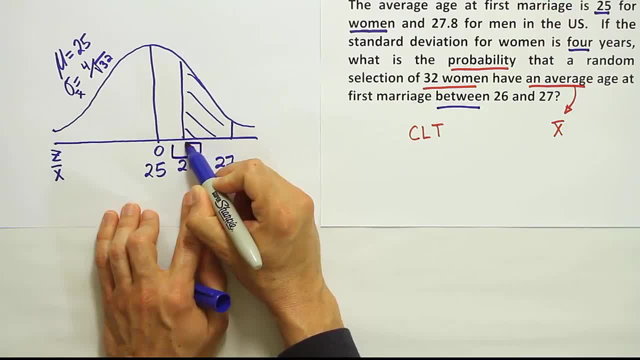 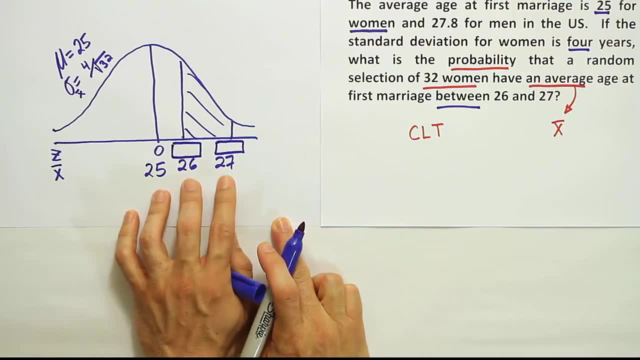 So my goal next is to go to my z table. Remember, once I have my drawing done and it's shaded, I'm supposed to go to my z table, But I can't go there until I have z scores to look up. I can't look up these ages. They're not z scores, So I have to convert them first to 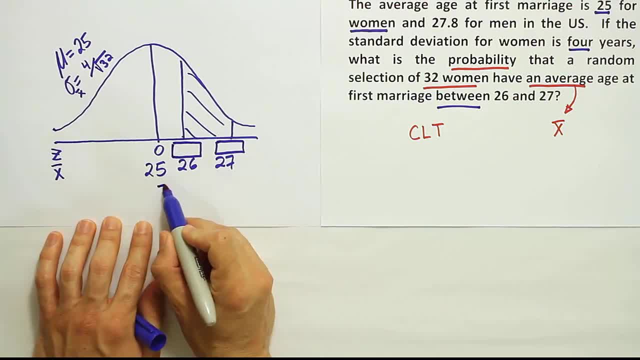 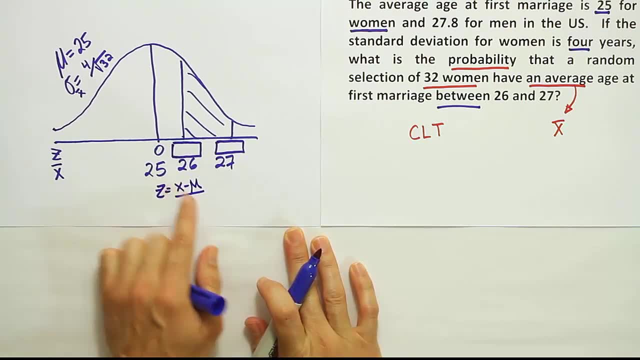 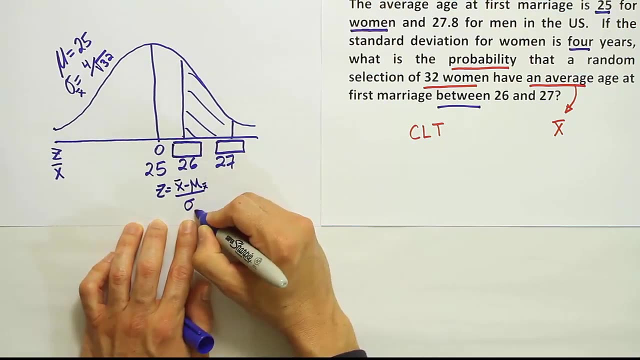 z scores. So let's do that first for the 26.. Remember that z is equal to x minus the mean over sigma, right? Well, here we have x bar minus the mean for x bar, minus sigma of x bar. But that's really just notation, right? I mean, you can plug that stuff in, But essentially 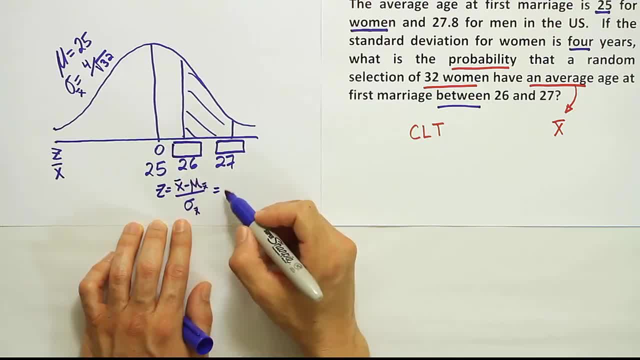 it doesn't really change what we've been doing since before. If I want to convert this number, 26,, I put 26 down, I take the mean from up here, 25.. And then I divide by this quantity 4 divided by the square root of 32.. Just be careful. 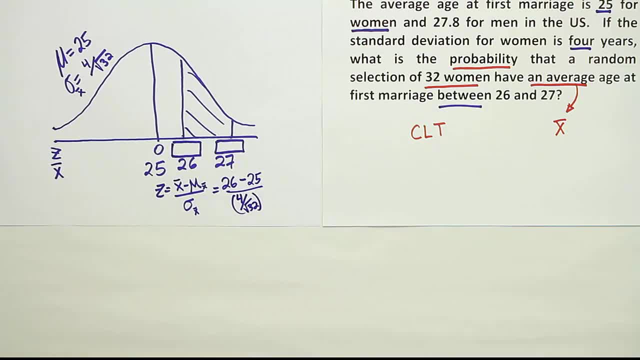 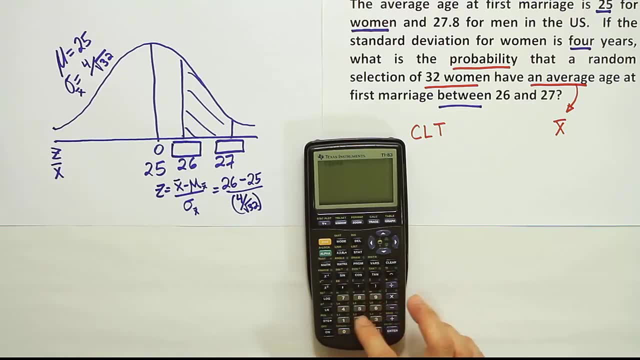 when you do that, If you do it in your calculator, put it in parentheses so you don't make a mistake. Let me show you how this would be done in your calculator. if you want to do it all at once in your calculator, You would actually use parentheses and say 26 minus. 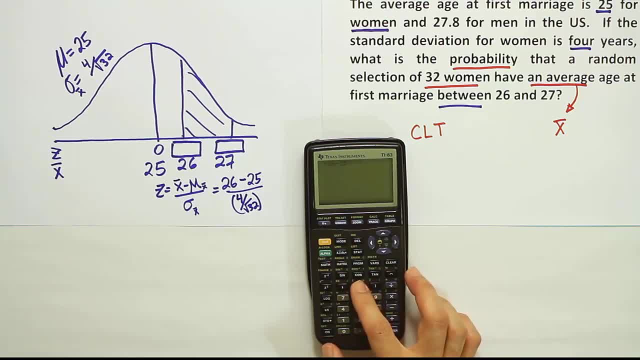 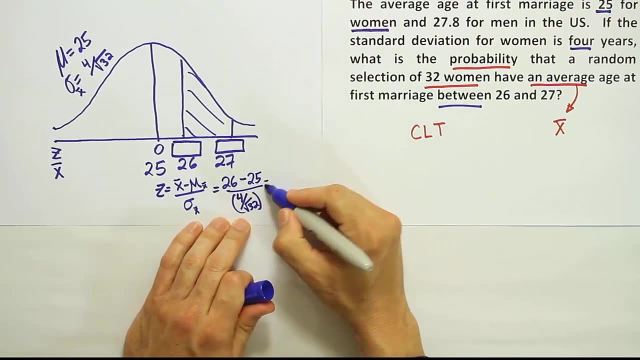 25, close the parentheses divided by open parentheses, 4 divided by the square root of 32.. Close that, Close it one more time And then you get the answer 1.41 when rounded off to two places. So we'll have the answer. 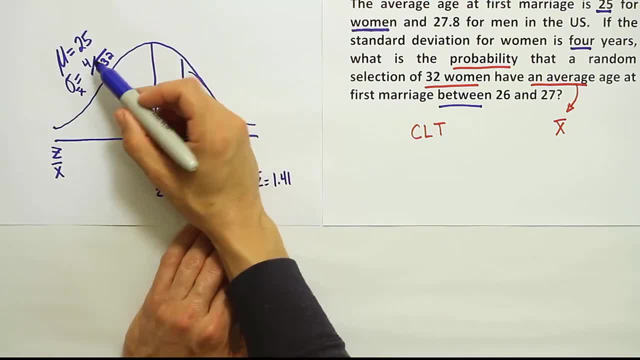 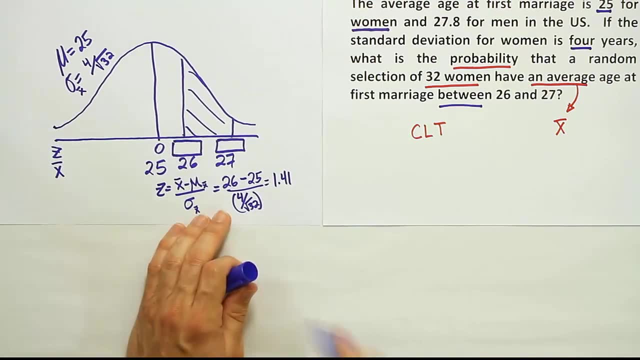 1.41.. An alternative way to do it is to just work out this as a decimal. Use several decimal places, put it at the bottom and you're good. okay, All right, so the first number is 1.41.. 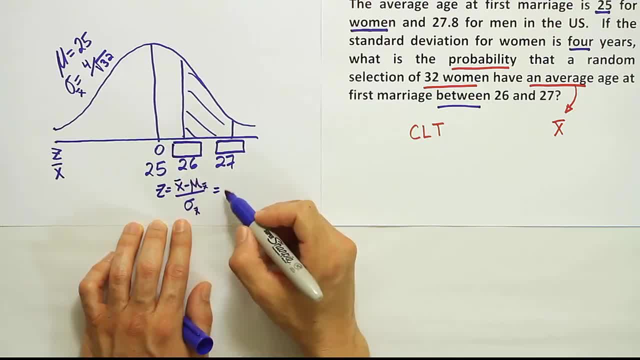 it doesn't really change what we've been doing since before. If I want to convert this number, 26,, I put 26 down, I take the mean from up here, 25.. And then I divide by this quantity 4 divided by the square root of 32.. Just be careful. 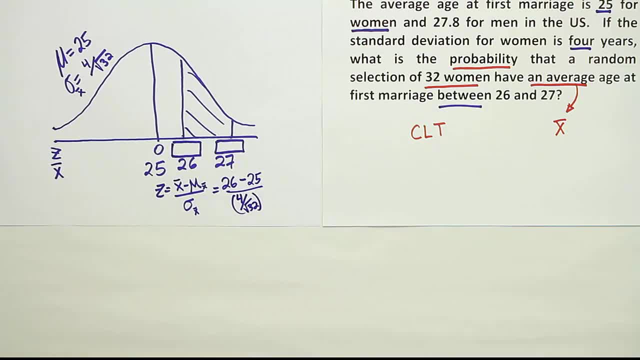 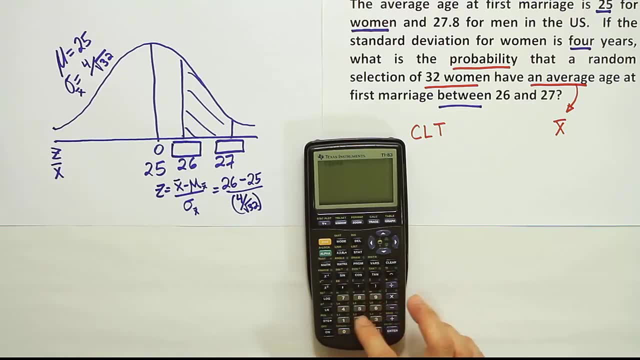 when you do that, If you do it in your calculator, put it in parentheses so you don't make a mistake. Let me show you how this would be done in your calculator. if you want to do it all at once in your calculator, You would actually use parentheses and say 26 minus. 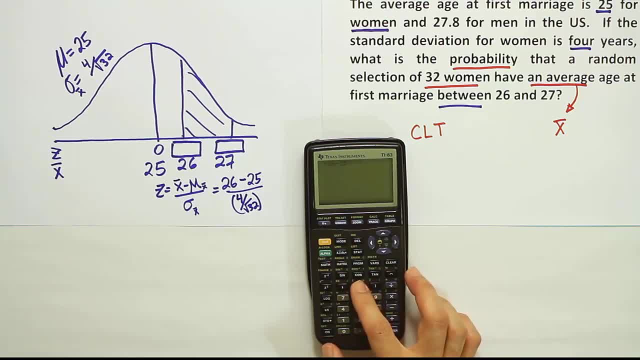 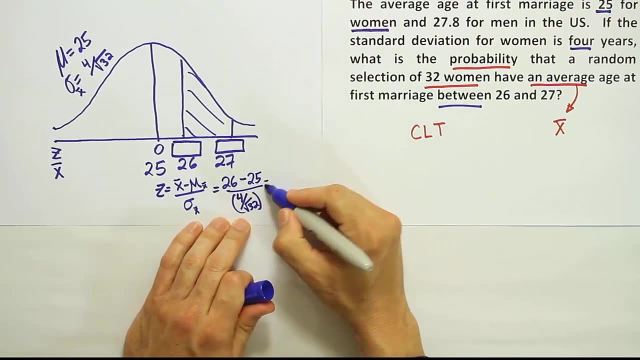 25, close the parentheses divided by open parentheses, 4 divided by the square root of 32.. Close that, Close it one more time And then you get the answer 1.41 when rounded off to two places. So we'll have the answer. 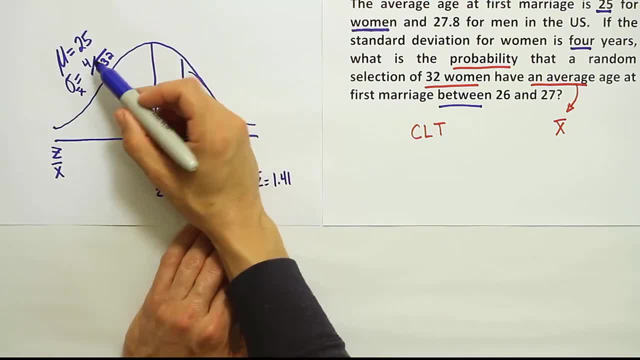 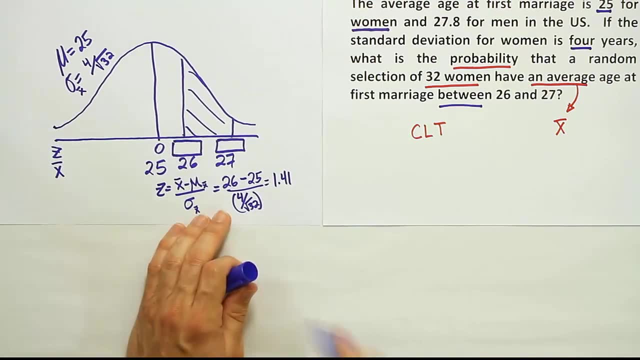 1.41.. An alternative way to do it is to just work out this as a decimal. Use several decimal places, put it at the bottom and you're good. okay, All right, so the first number is 1.41.. 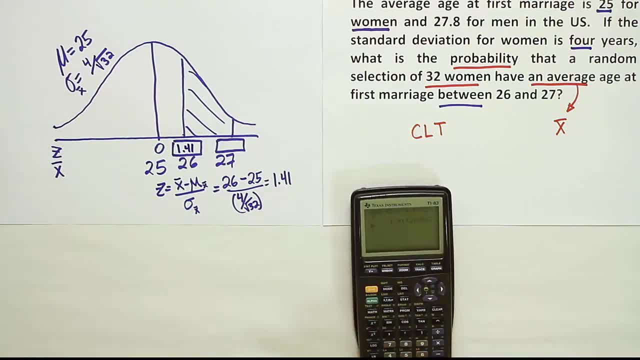 The second z-score is going to be 27 minus 25.. Of course that gives you 2. You don't have to work that out in your calculator. But at this point then we just divide by 4, divided by the square root of 32. And then we're good, And then we're good, And then 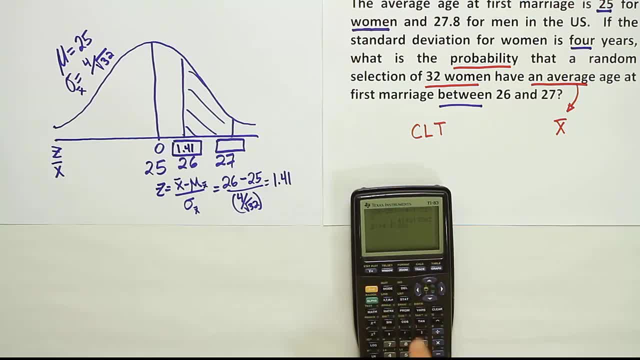 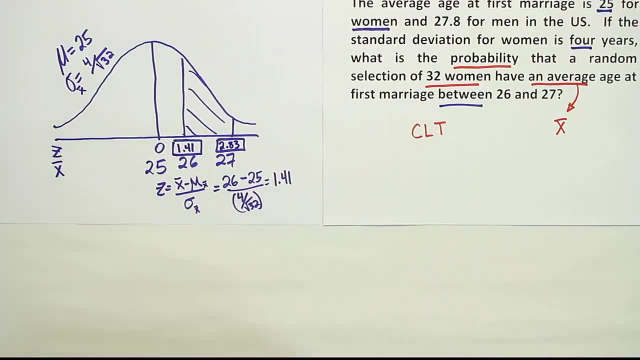 Okay, So now you have your two z-scores. We're going to look them up. Remember, when we look up 1.41, we're going to get the area from here to here. That's not the area we want. 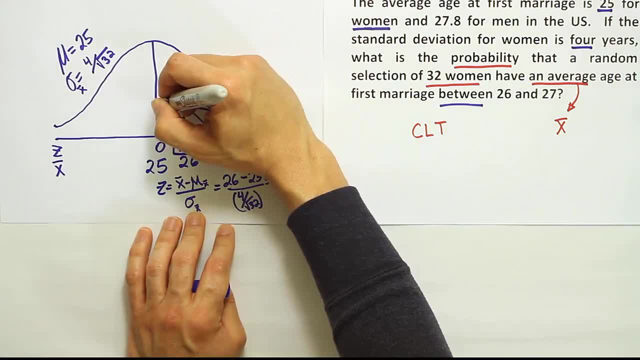 When we look up to 2.83, we're going to get the area from here all the way to there, which is not the area we want either. It's all of what we want, plus a little extra. So remember, when you have this kind of a drawing, you have to subtract that next one into the square. 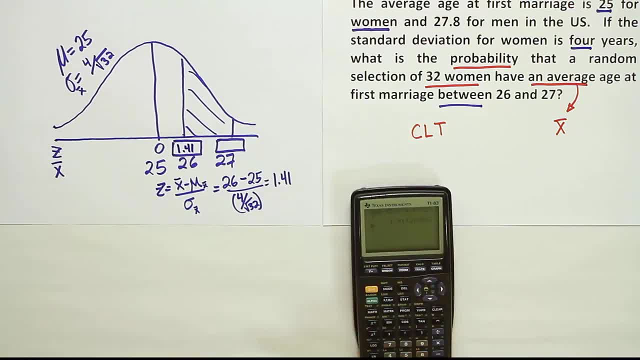 The second z-score is going to be 27 minus 25.. Of course that gives you 2. You don't have to work that out in your calculator. But at this point then we just divide by 4, divided by the square root of 32.. And then we're good, We're good, We're good, We're. 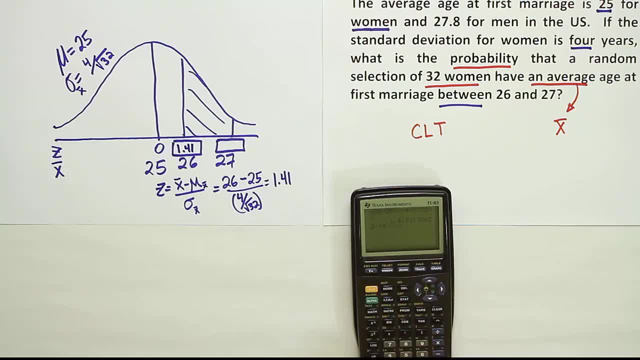 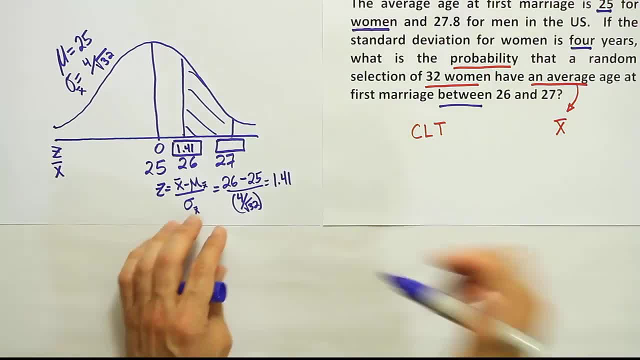 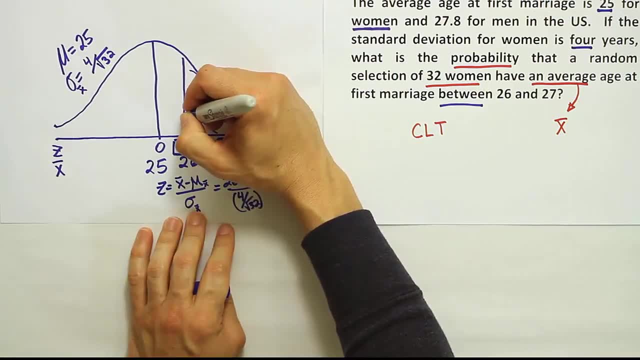 you end up with the answer 2.83.. 2.83.. Okay, so now you have your two z-scores. We're going to look them up. Remember, when we look up 1.41, we're going to get the area from here. 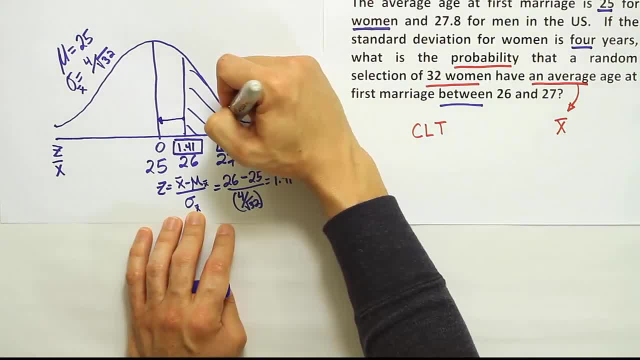 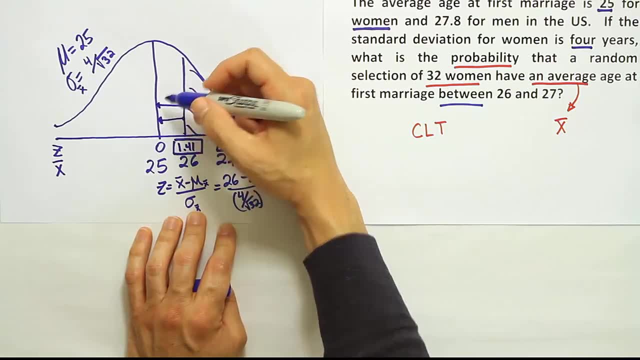 to here. That's not the area we want. And when we look up 2.83, we're going to get the area from here all the way to there, which is not the area we want either. It's all of what we want, plus a little extra. So remember, when you have this kind of a drawing, you 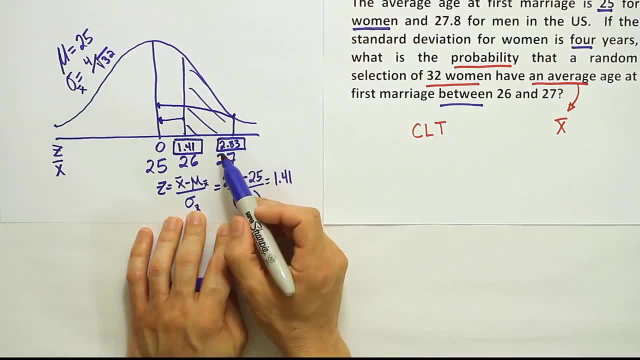 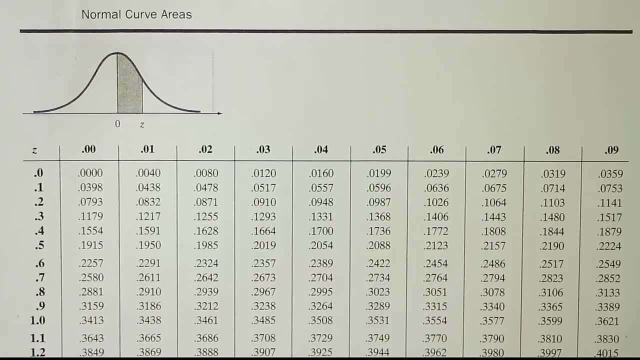 have a little extra. So remember, when you have this kind of a drawing you have a little have to subtract the two results that you get from the Z table. So let's go to the table now and look up 2.83 and 1.41.. So in this problem we're looking up two Z. 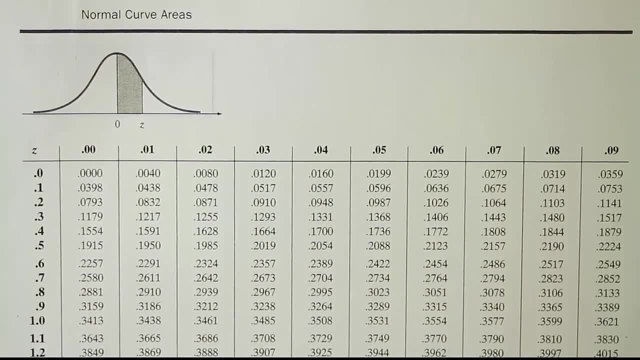 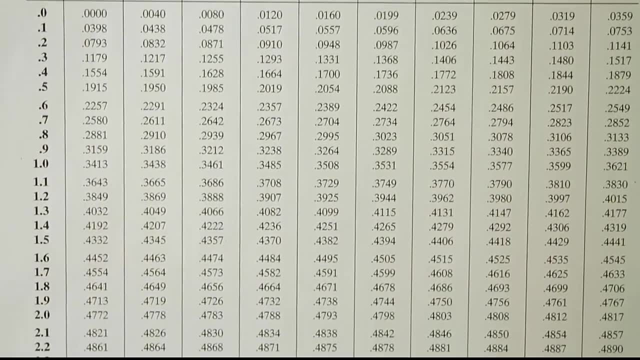 scores. We're looking up 2.83 and 1.41.. Let's go get the 2.83 first. Let's move the table down. here I'm looking for the first two digits, 2.8.. So there, I see the. 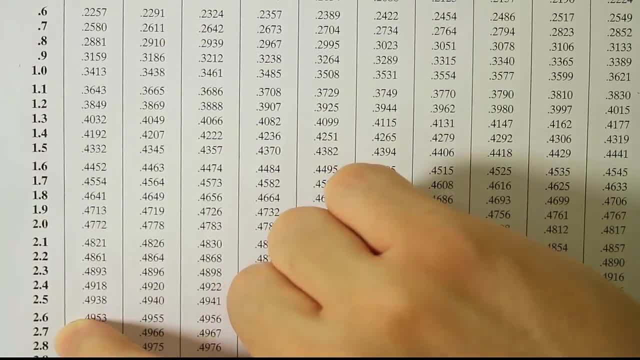 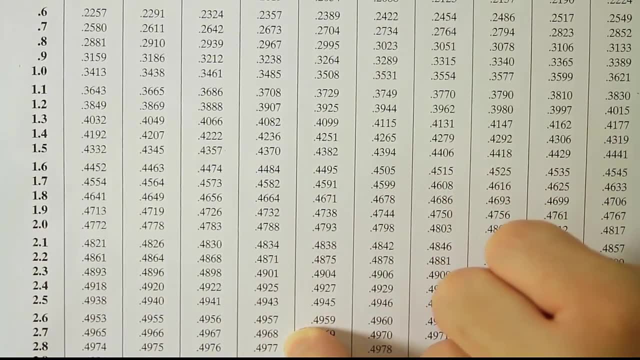 2.8 row. I'm going to go over until I get to 3.. So it's 2.80,, 2.81,, 2.82,, 2.83.. So the first number we get is 0.4977.. So that first area is 0.4977.. All right, so now we 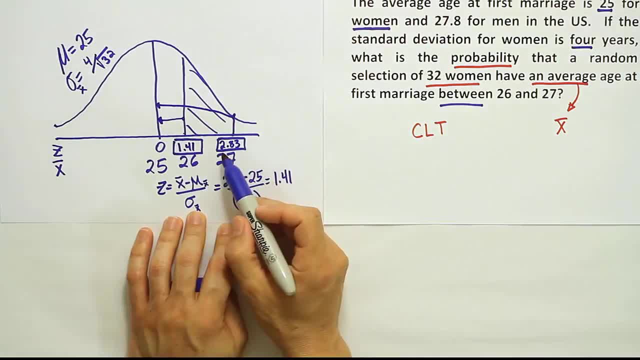 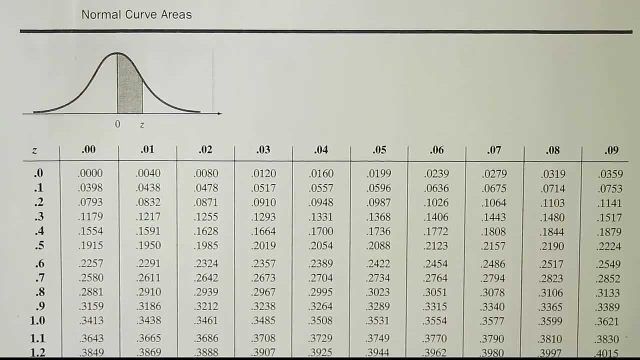 square root. If you subtract that, then what you get in particular is 32 minus 27.. and if have to subtract the two results that you get from the Z table. So let's go to the table now and look up 2.83 and 1.41.. So in this problem we're looking up two Z. 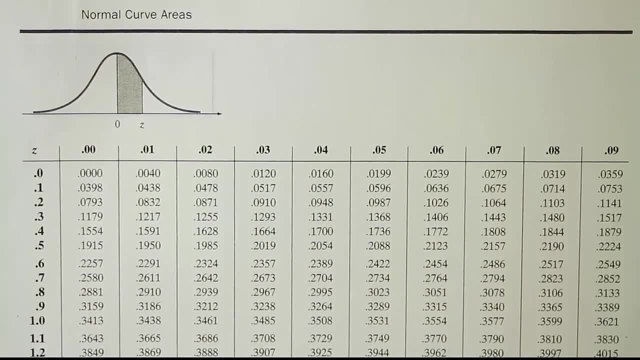 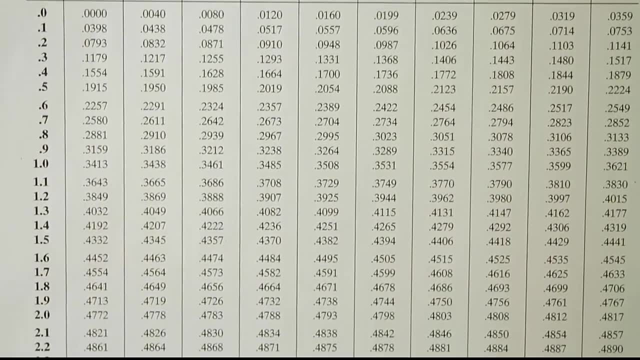 scores. We're looking up 2.83 and 1.41.. Let's go get the 2.83 first. Let's move the table down. here I'm looking for the first two digits, 2.8.. So there, I see the. 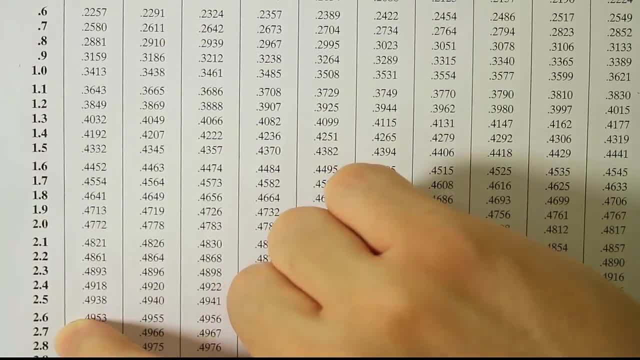 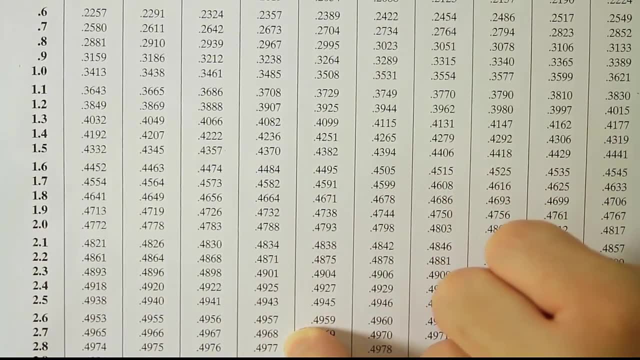 2.8 row. I'm going to go over until I get to 3.. So it's 2.80,, 2.81,, 2.82,, 2.83.. So the first number we get is 0.4977.. So that first area is 0.4977.. All right, so now we 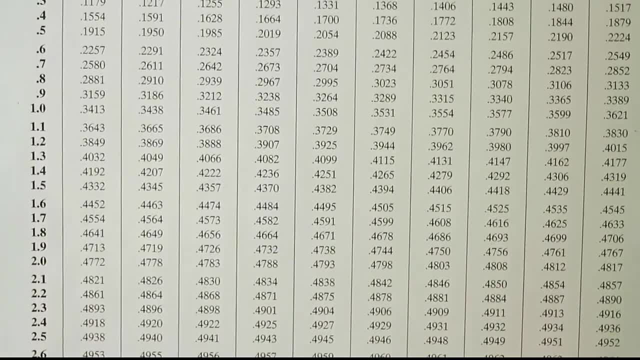 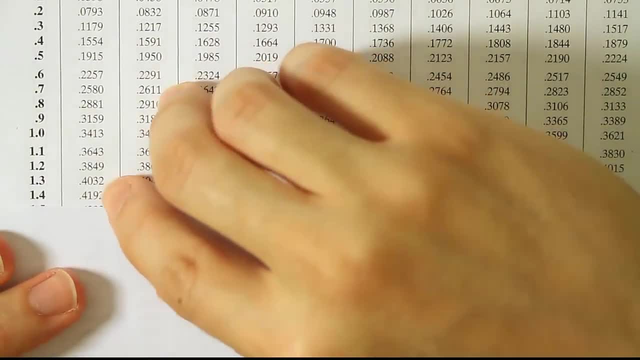 have to look up 1.41.. Let's bring the table back down And we can see that 1.4 is about here And that first position is going to be 1.40 and then 1.41.. So we're going to. 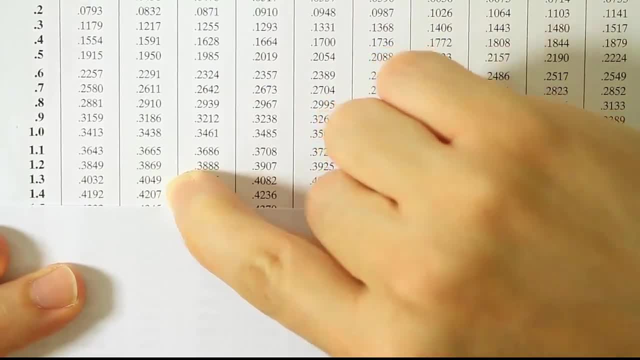 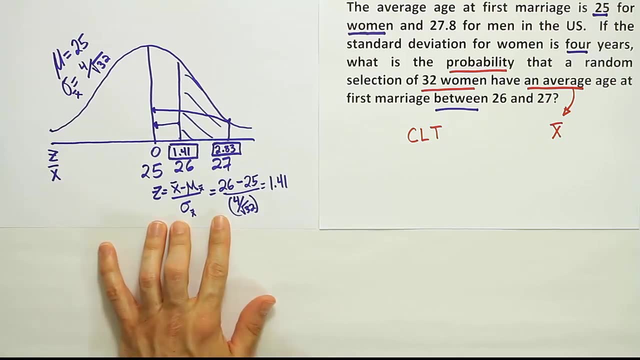 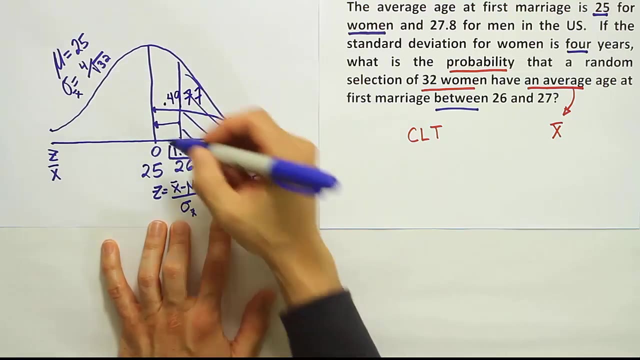 have the answer: 0.4207.. Okay, so let's put our two probabilities now on our drawing, 2.83 gave us 0.4977.. And the smaller of the two, the 1.41, gave us 0.4207.. So, in order. 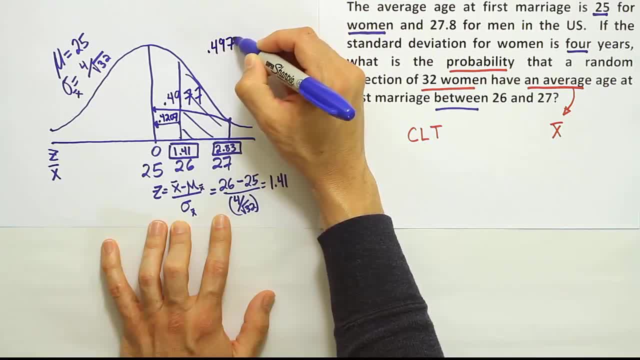 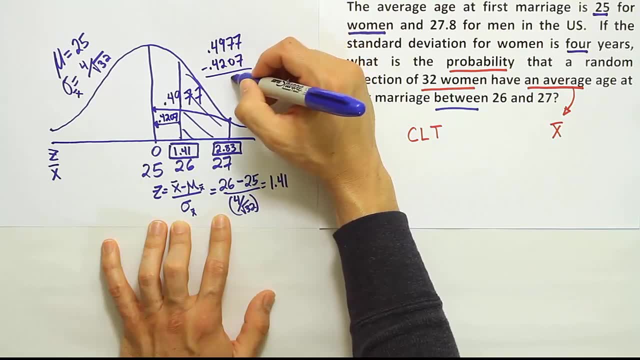 to get our final answer, we have to subtract those, So 0.4977 minus 0.4207.. If I do the subtraction here, I get 0, here, 7.. 2 from 9 is also 7.. And then 0 again. So. 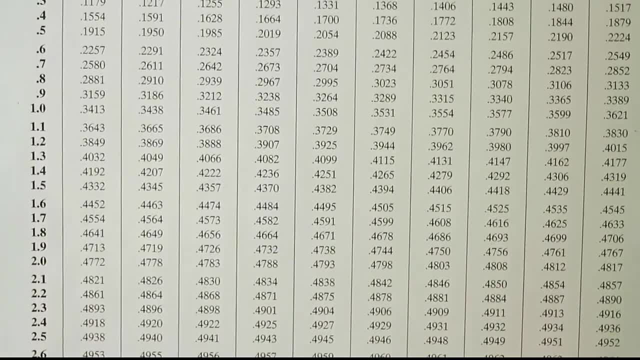 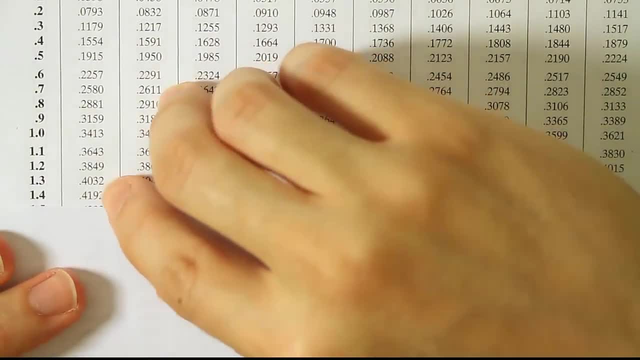 have to look up 1.41.. Let's bring the table back down And we can see that 1.4 is about here And that first position is going to be 1.40 and then 1.41.. So we're going to. 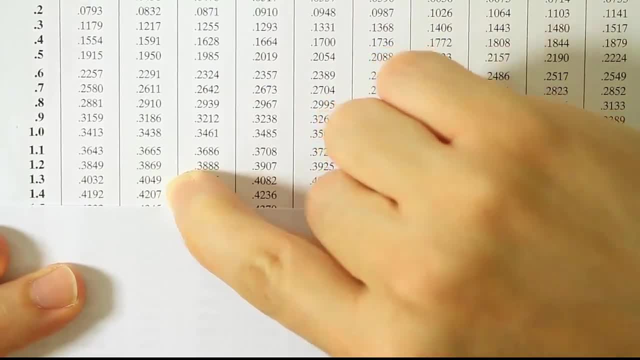 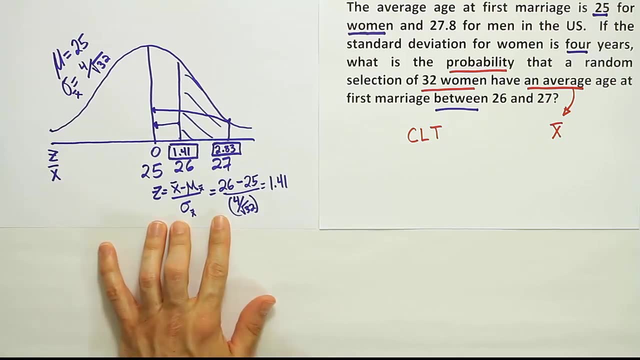 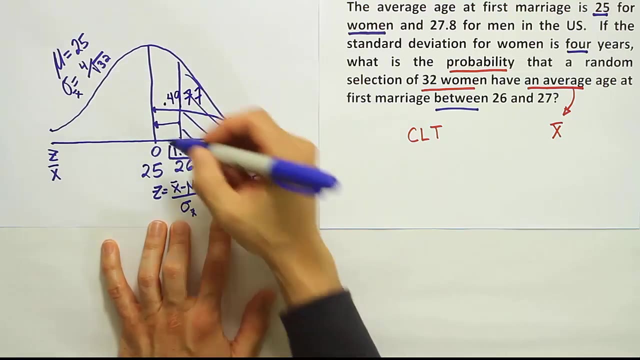 have the answer: 0.4207.. Okay, so let's put our two probabilities now on our drawing, 2.83 gave us 0.4977.. And the smaller of the two, the 1.41, gave us 0.4207.. So, in order. 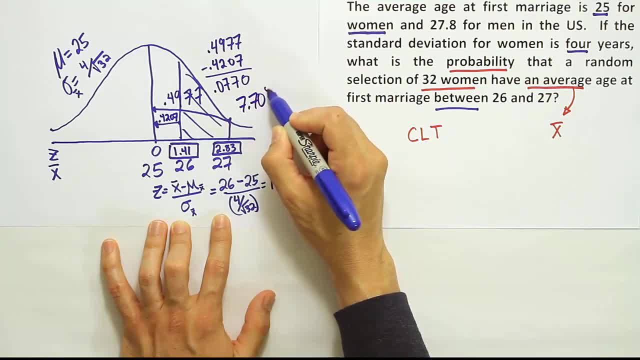 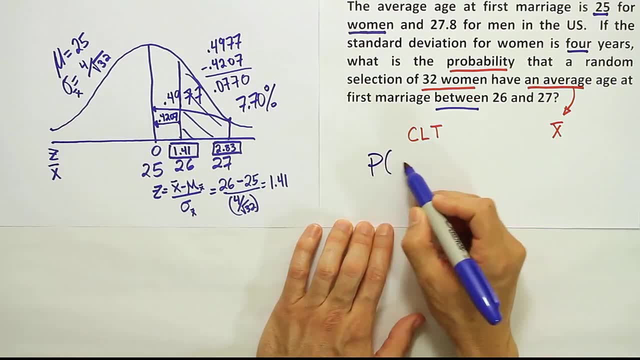 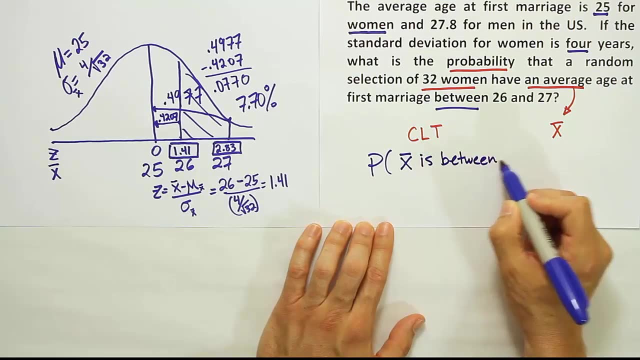 we get the answer 7.70% or 0.0770 as a decimal. All right, so our final answer is: the probability that the average height is between 26 and 27 is equal to 7.77.. So that's going to be. 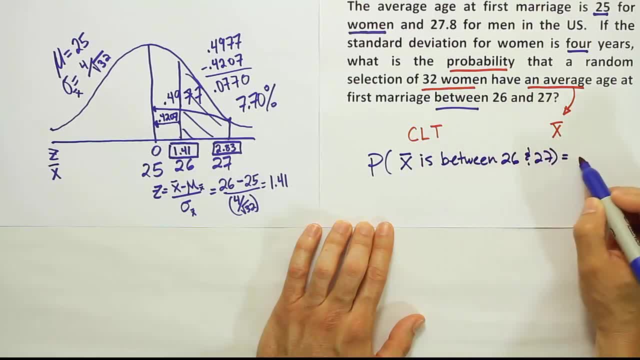 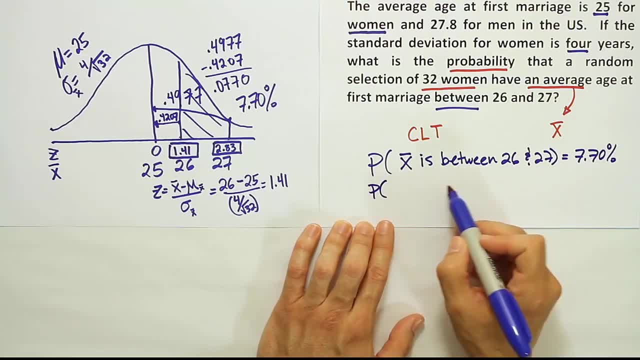 going to be 7.77.. So that's going to be 7.77. Another way to write it would be to say: the probability that x bar is less than 27, but greater than 26 is equal to 7.70%. 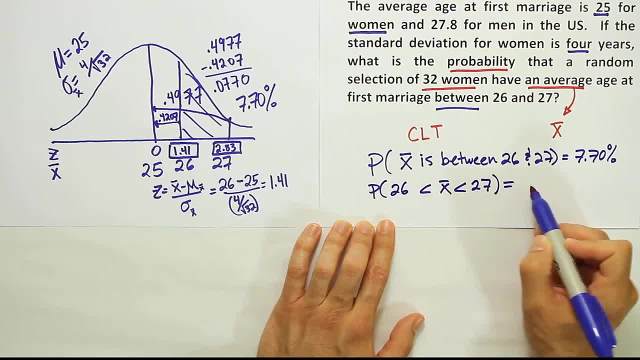 Another way to write it would be to say: the probability that x bar is less than 27 but greater than 26 is equal to 7.70%.